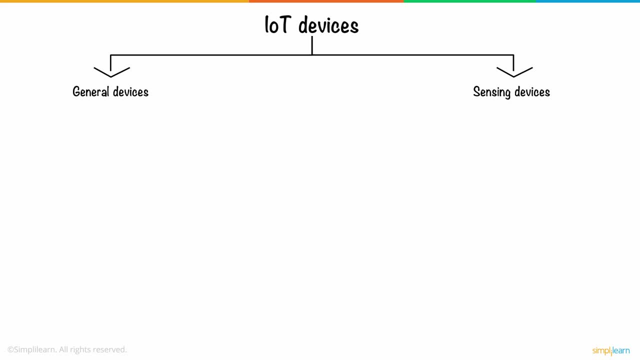 classified into General Devices and Sensing Devices. The General Devices are the main components of the data processing system. They are the main components of the data processing hub and information exchange. They are connected either by wired or wireless interfaces. Home appliances are a classic example of such devices. The Sensing Devices, on the other hand, 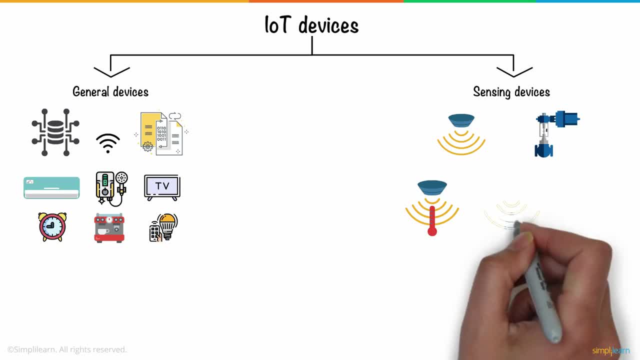 include sensors and actuators. They measure the temperature, humidity, light intensity and other parameters. These IoT devices are connected to the network with the help of gateways. These gateways, or processing nodes, process the information collected from the sensors and transfer it to the cloud. These gateways or processing nodes process the 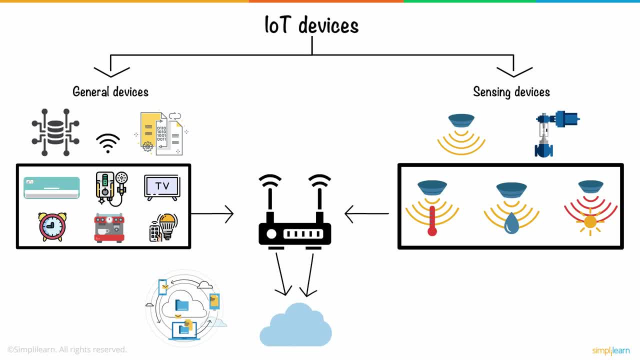 information collected from the sensors and transfer it to the cloud. The cloud acts as both the storage and processing unit. Actions are performed on the collected data for further learning and inferences. Wired and wireless interfaces like Wi-Fi, Bluetooth, ZigBee. 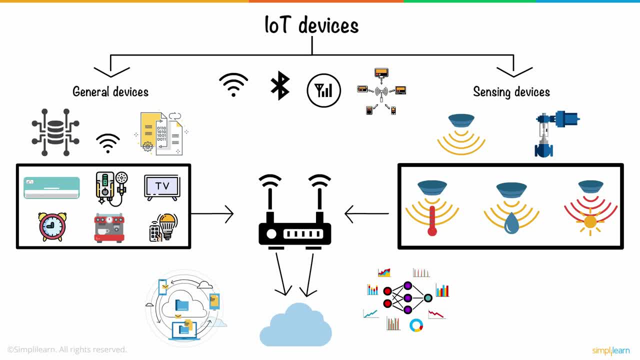 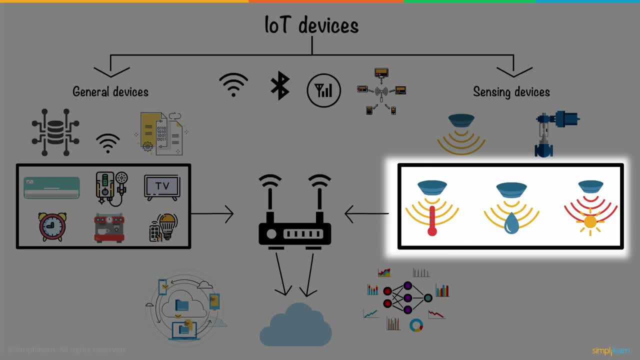 GSMs and so on, are used to provide connectivity. To ensure its ubiquity, applications need to support a diverse set of devices and communication protocols, from tiny sensors capable of sensing and reporting the desired factor to powerful back-end servers that are utilized for 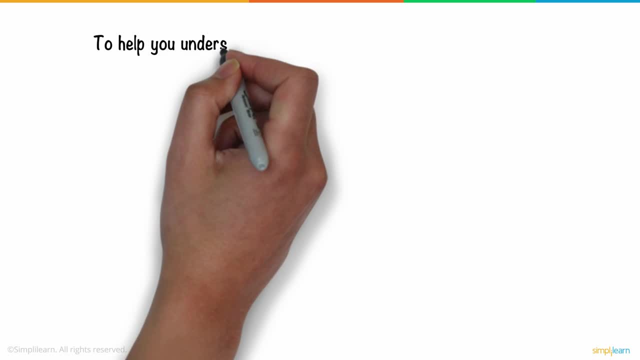 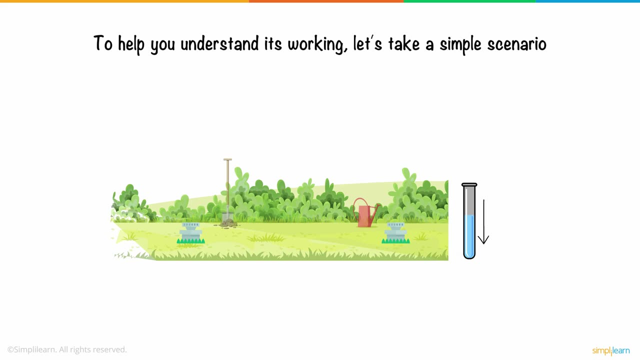 data analysis and knowledge extraction. To help you understand its working, let's take a simple scenario. Let's suppose you want to water your garden every time the moisture level in the soil drops. Instead of doing it manually, you could automate it using IoT. 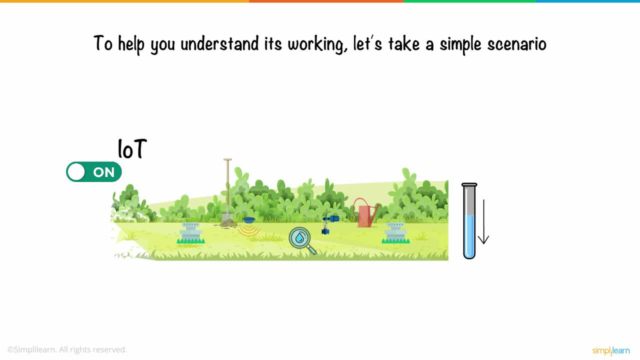 The sensors and actuators installed gauge the soil for its moisture. This information is sent to the IoT gateway with the help of communication protocols like MQTT or HTTP. The gateway significantly aggregates data and feeds it to the cloud with the help of Wi-Fi LAN Once the moisture level drops. 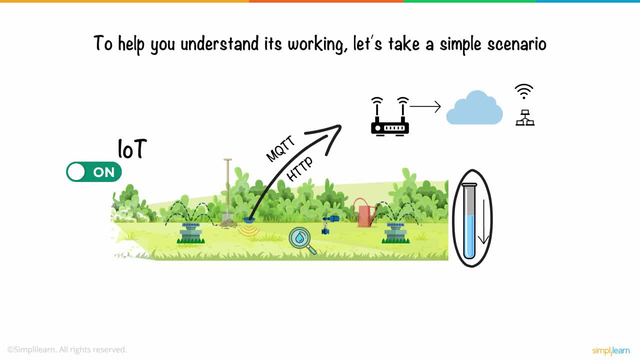 the system is immediately triggered and the sprinklers are turned on. However, with the information stored in the cloud, a detailed analysis, like the time of the day the sprinkler was turned on, the rate at which the moisture in the soil reduces, and so on. 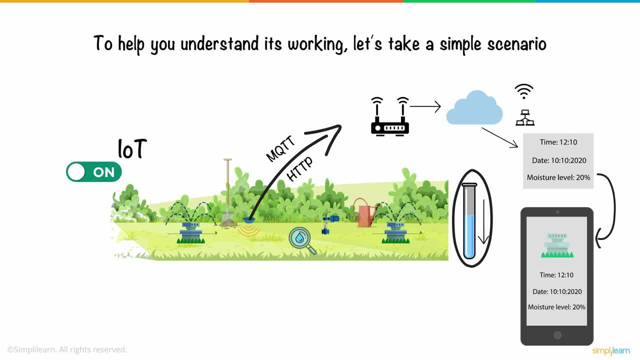 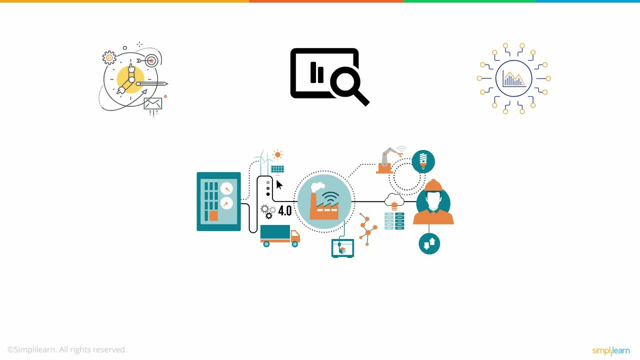 can be done and the report could be sent over to you on your smartphone over an app. With the improved response, monitoring and analytical capabilities, IoT is being adopted in almost all industries and domains. With the improved response, monitoring and analytical capabilities, IoT is being adopted in almost all industries and domains. 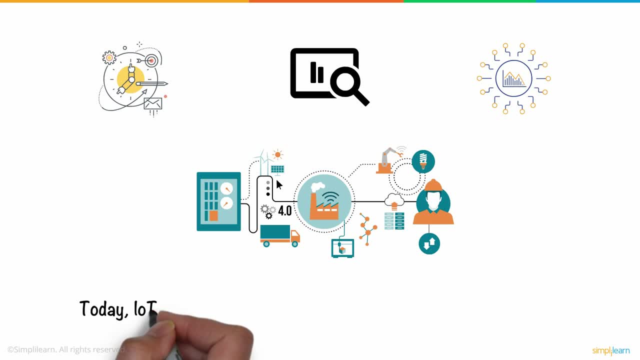 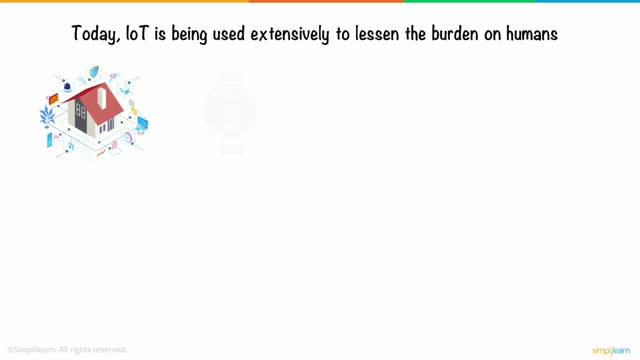 With the improved response, monitoring and analytical capabilities. IoT is being adopted in almost all industries and domains, Opening doors to endless applications. Today, IoT is being used extensively to lessen the burden on humans. To name a few, IoT is deployed for smart homes, wearables, watches and bracelets, smart cars. 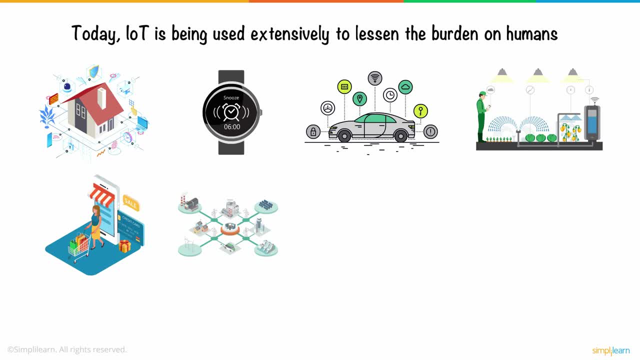 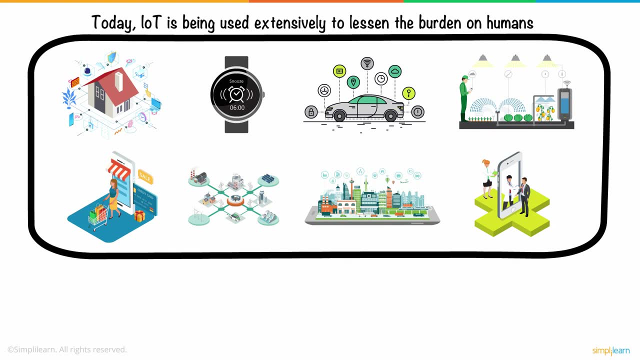 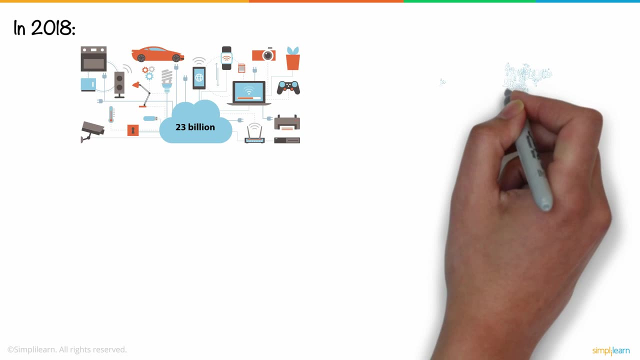 smart farming, smart retail, smart grids, smart city and smart healthcare. With such a wide spectrum of applications, the future of IT looks more promising than ever before. In 2018,, there were about 23 billion connected devices, which was more than double the world population, According to experts. 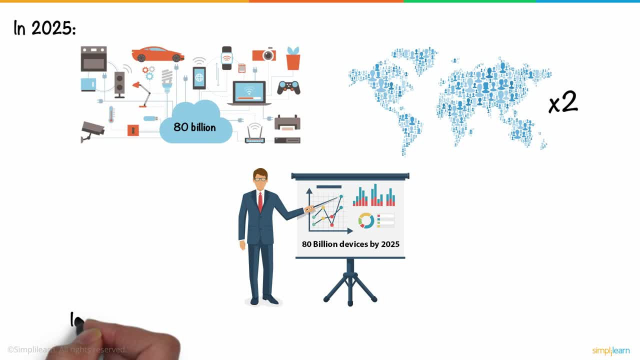 there will be over 80 billion devices by 2025.. IoT is a vision to connect all devices with the power of the internet, Always learning and always growing. Now that you have a picture of what IoT is, here's a simple question for you. 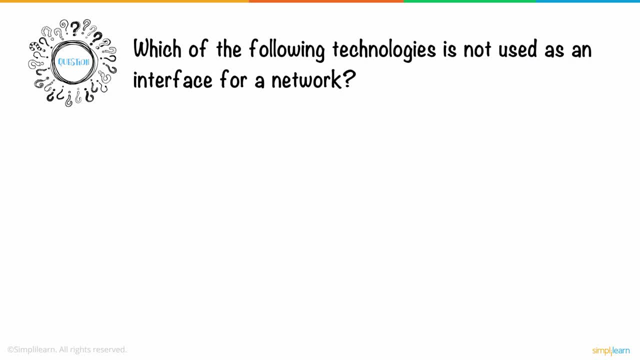 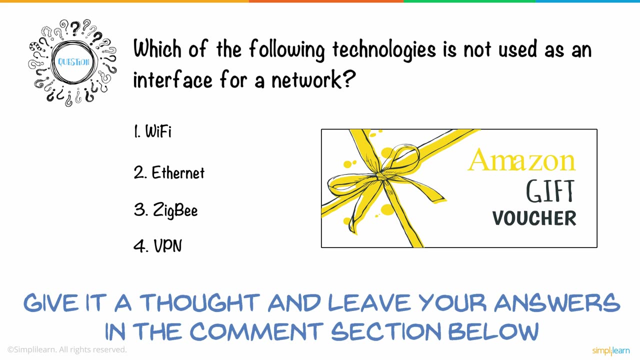 Which of the following technologies is not used as an interface for a network: 1. Wi-Fi, 2. Ethernet. 3. Zigbee, 4. VPN. Give it a thought and leave your answers in the comment section below. Three lucky winners will receive Amazon gift vouchers. 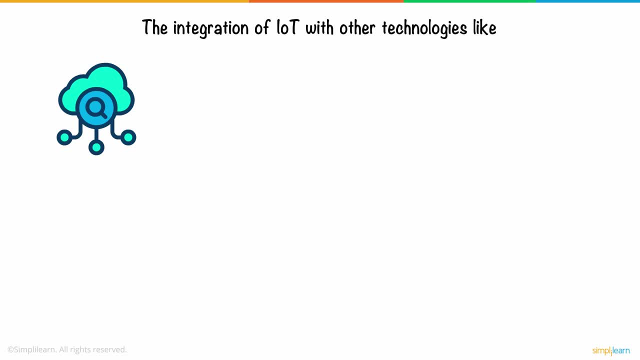 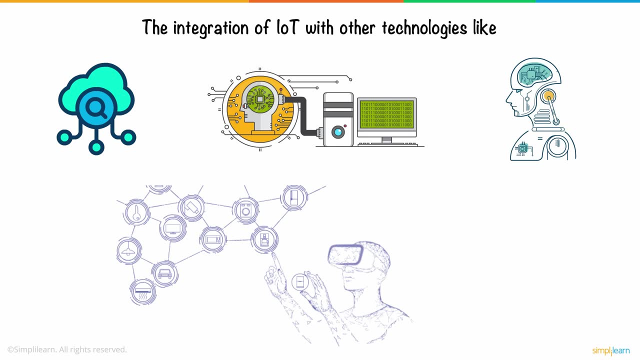 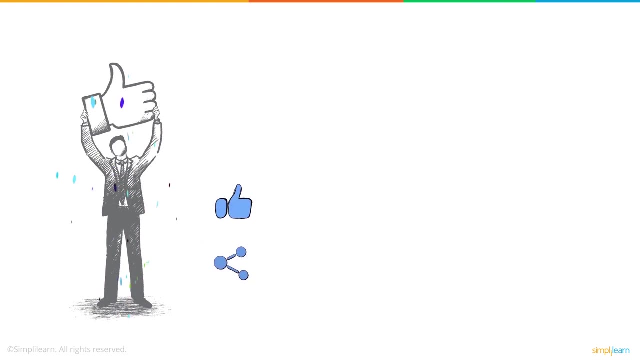 The integration of IoT with other technologies like cloud computing, machine learning and artificial intelligence is paving the way for many new and exciting innovations, And that is the Internet of Things for you. in short, If you enjoyed this video, a thumbs-up would be really appreciated. 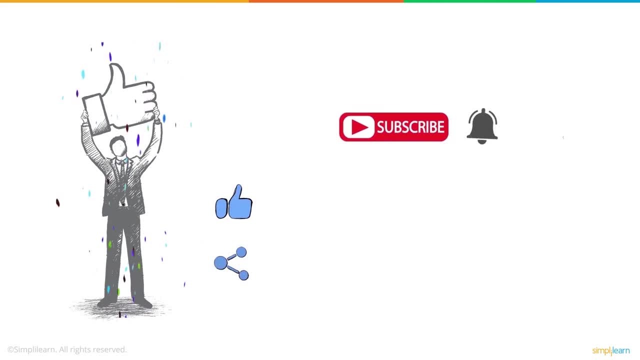 Don't forget to subscribe to the Simply Learn channel and hit the bell icon to never miss an update on the latest trending technologies.